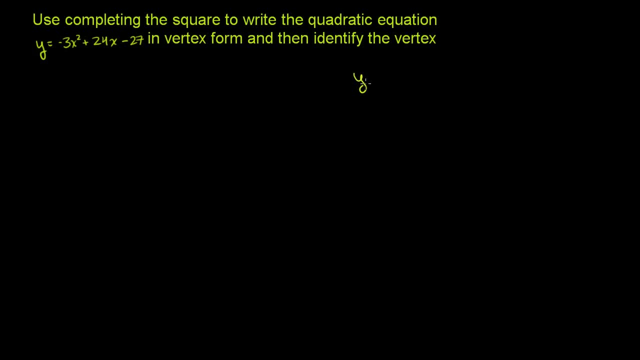 rewrite. we algebraically manipulate it, so it's in the form: y is equal to a times x minus b, squared plus c. We want to get the equation into this form right here. This is vertex form right there, And once you have it in vertex form, you'll see that you can. 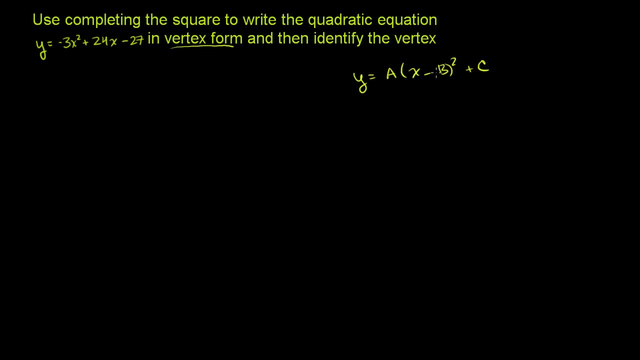 identify the x value of the vertex as what value will make this expression equal to 0.. So in this case it would be b And the y value of the vertex. if this is equal to 0, then the y value is just going to be c. 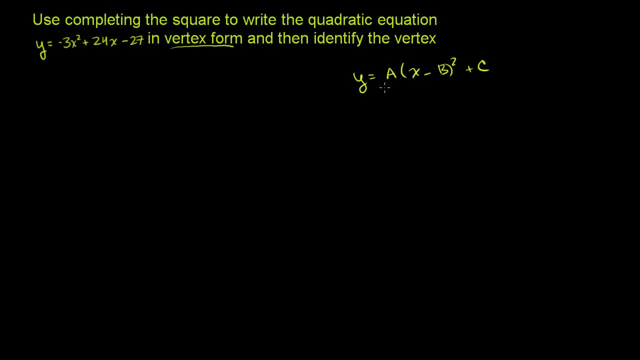 And we're going to see that and we're going to understand why that is the vertex, why this vertex form is useful. So let's try to manipulate this equation to get it into that form. So if we just rewrite it, the first thing that immediately. 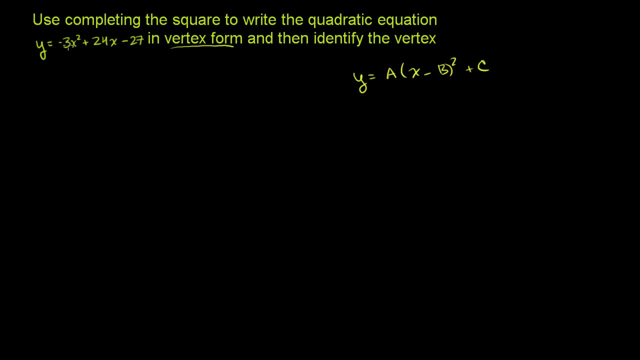 jumps out, at me at least, is that all of these numbers are divisible by negative 3.. And I just always find it easier to manipulate an equation if I have a 1 coefficient out in front of the x squared. So let's just factor out a negative 3 right from the get. 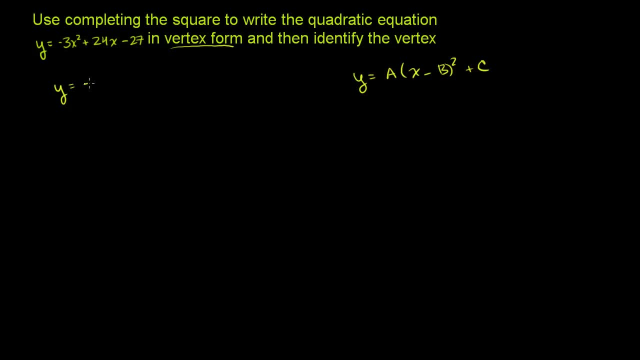 go. So we can rewrite this as: y is equal to negative 3 times x squared minus 8x. 24 divided by negative 3 is negative 8, plus 9.. Negative 27 divided by negative 3 is positive 9.. 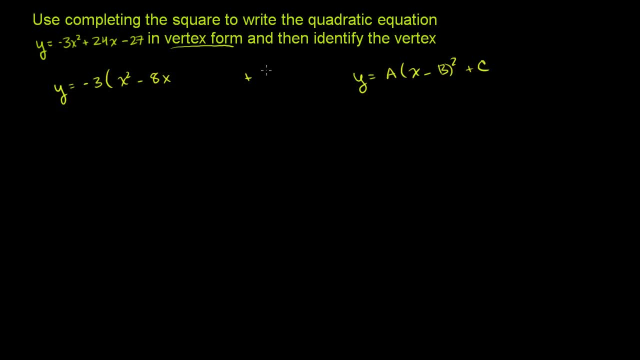 And let me write the positive 9 out here, And you're going to see in a second why I'm doing that. Now we want to be able to express part of this expression as a perfect square. That's what vertex form does for us. 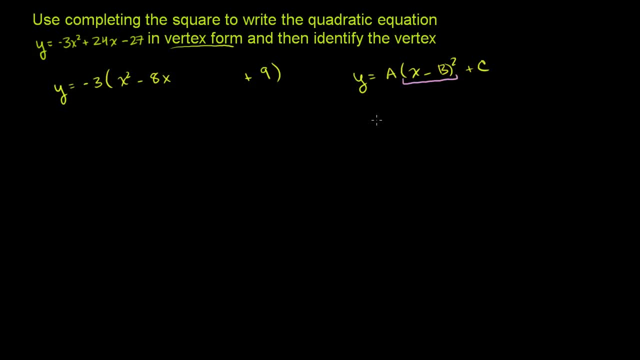 We want to be able to express part of this expression as a perfect square. Now, how can we do that? Well, we have an x squared minus 8x. So if we had a positive 16 here, because, well, just, 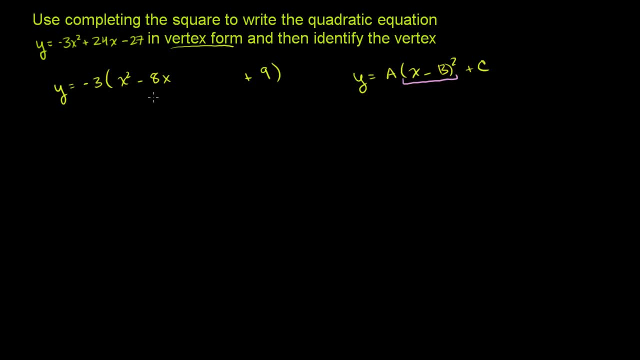 think about it this way: If we had negative 8, you divide it by 2, you get negative 4.. You square that: it's positive 16.. So if you had a positive 16 here, this would be a perfect. 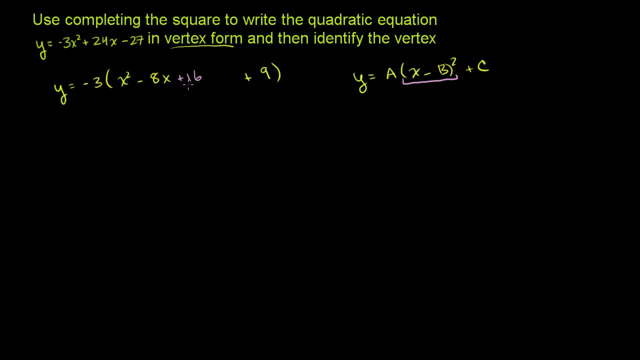 square. this would be x minus 4 squared. But you can't just willy nilly add a 16 there. You could either have to add a form out to the other side and you would have to scale it by the negative 3 and all of that. 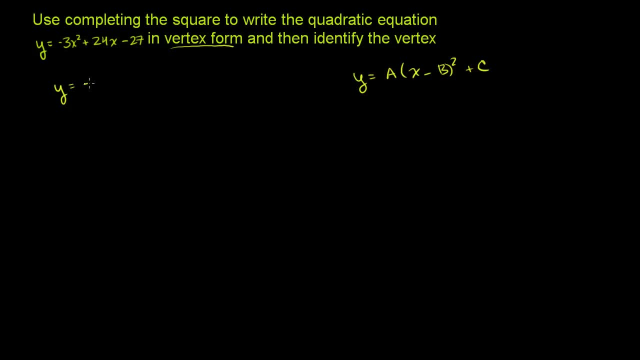 go. So we can rewrite this as: y is equal to negative 3 times x squared minus 8x. 24 divided by negative 3 is negative 8, plus 9.. Negative 27 divided by negative 3 is positive 9.. 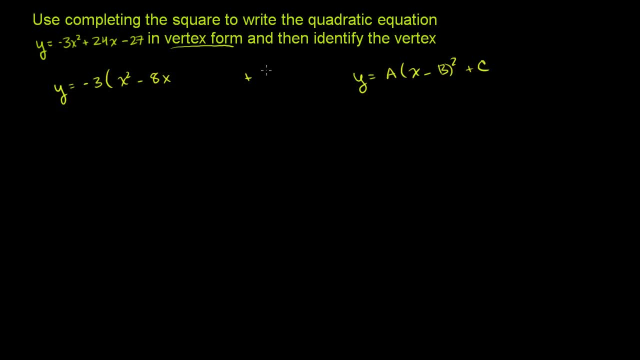 And let me write the positive 9 out here, And you're going to see in a second why I'm doing that. Now we want to be able to express part of this expression as a perfect square. That's what vertex form does for us. 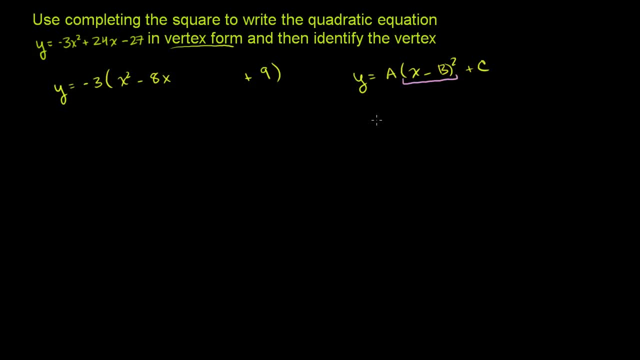 We want to be able to express part of this expression as a perfect square. Now, how can we do that? Well, we have an x squared minus 8x. So if we had a positive 16 here, because, well, just, 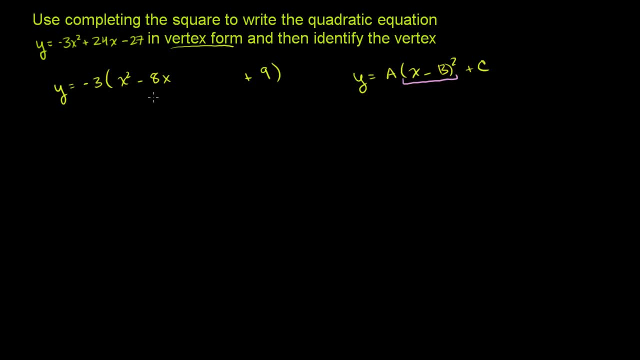 think about it this way: If we had negative 8, you divide it by 2, you get negative 4.. You square that: it's positive 16.. So if you had a positive 16 here, this would be a perfect. 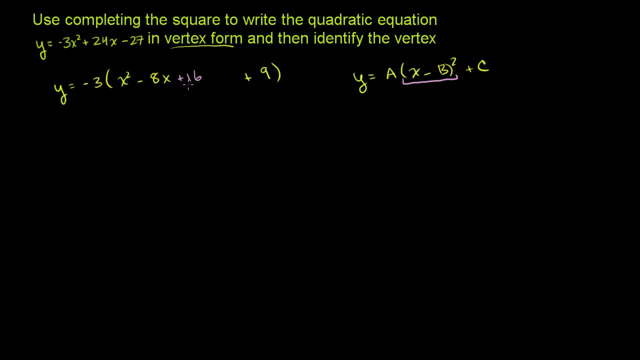 square. this would be x minus 4 squared. But you can't just willy nilly add a 16 there. You could either have to add a form out to the other side and you would have to scale it by the negative 3 and all of that. 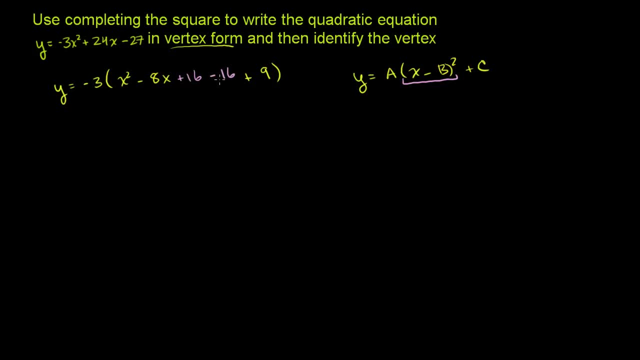 Or you can just subtract a 16 right here. I haven't changed the expression. I'm adding a 16, subtracting a 16.. I've added a 0. I haven't changed it, But what it allows me to do is express this part of the. 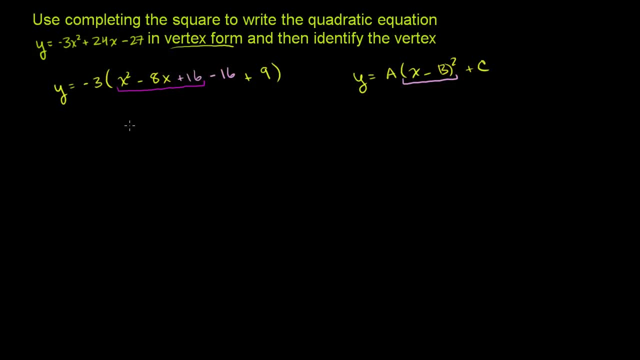 equation as a perfect square. That right, there is x minus 4 squared. And if you're confused, how did I know 16?? Just think I took negative 8, I divided it by 2, I got negative 4.. 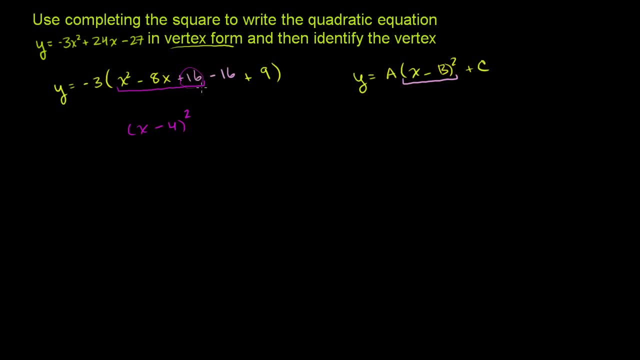 And then I squared negative 4.. This is negative 4 squared right there, And then I had to subtract that same amount, so I don't change the equation. So that part is x minus 4 squared, And then we still have this negative 3 hanging out there. 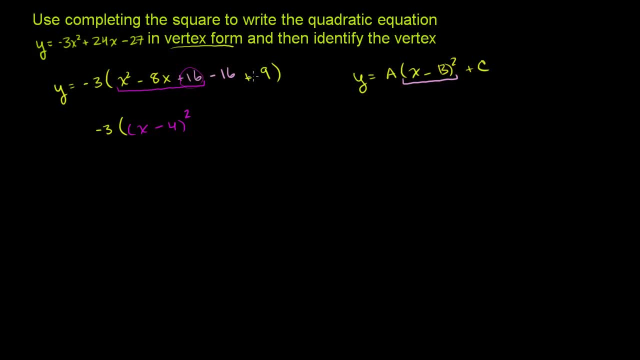 We still have that negative 3.. And then we have negative 16 plus 9, which is negative 7.. So we're almost there. We have y is equal to negative 3 times this whole thing. Not quite there. To get it there, we just multiply negative 3, we. 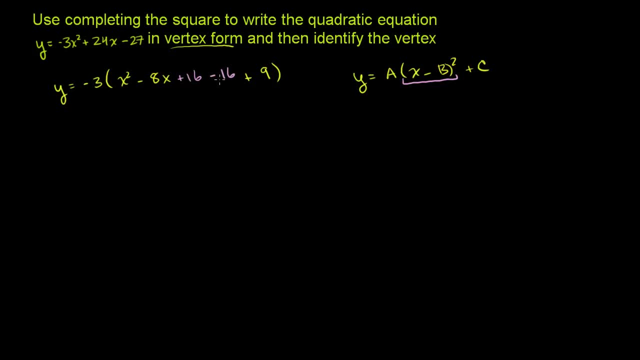 Or you can just subtract a 16 right here. I haven't changed the expression. I'm adding a 16, subtracting a 16.. I've added a 0. I haven't changed it, But what it allows me to do is express this part of the. 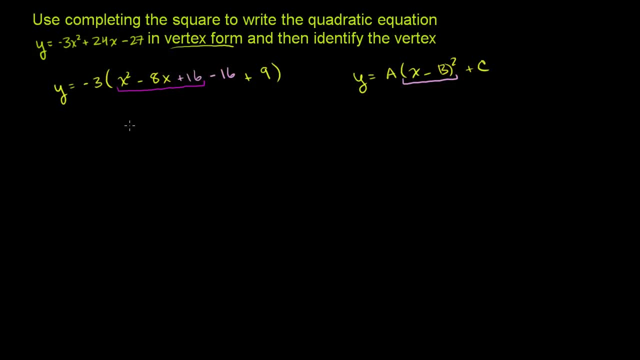 equation as a perfect square. That right, there is x minus 4 squared. And if you're confused, how did I know 16?? Just think I took negative 8, I divided it by 2, I got negative 4.. 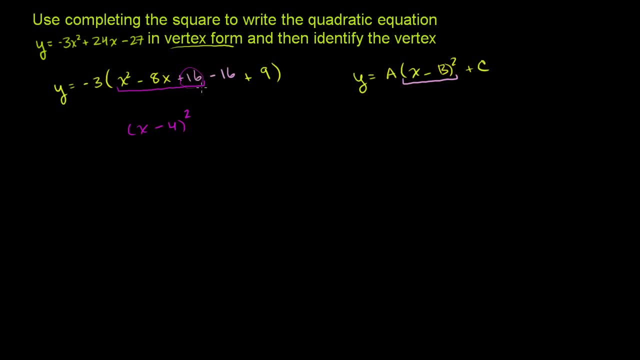 And then I squared negative 4.. This is negative 4 squared right there, And then I had to subtract that same amount, so I don't change the equation. So that part is x minus 4 squared, And then we still have this negative 3 hanging out there. 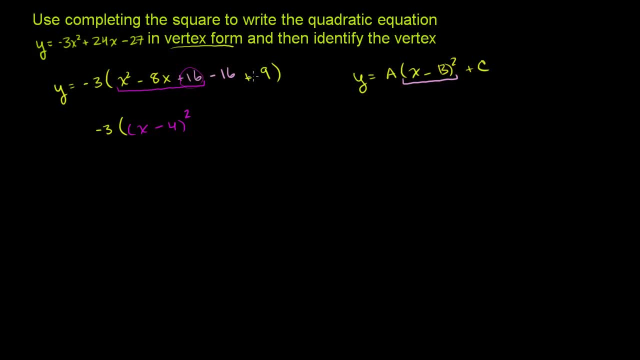 We still have that negative 3.. And then we have negative 16 plus 9, which is negative 7.. So we're almost there. We have y is equal to negative 3 times this whole thing. Not quite there. To get it there, we just multiply negative 3, we. 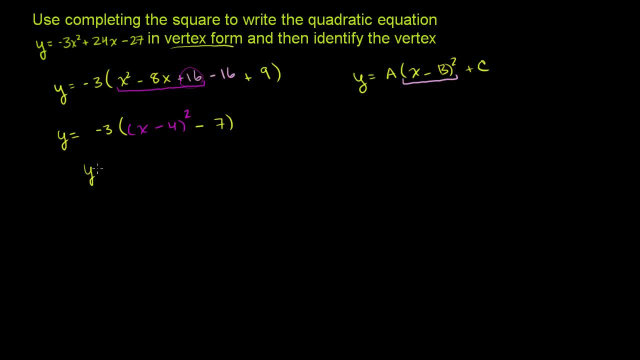 distribute the negative 3.. On to both of these terms. So we get: y is equal to negative 3 times x minus 4 squared, and negative 3 times negative. 7 is positive 21. So we have it in our vertex form. 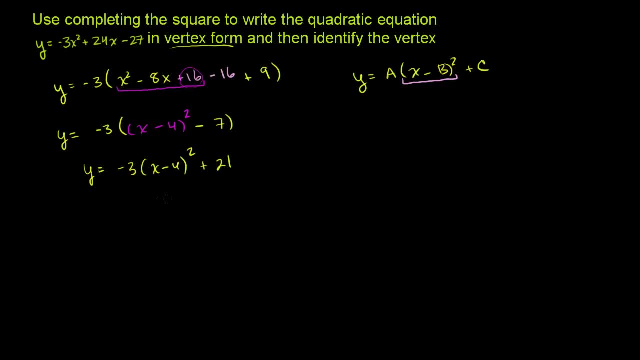 We're done that, And if you want to think about what the vertex is, I told you how to do it. you say: well, what's the x value that makes this equal to 0?? Well, in order for this term to be 0, x minus 4 has to be. 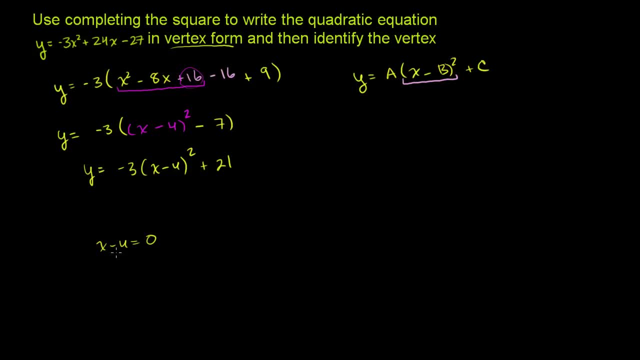 equal to 0. x minus 4 has to be equal to 0, or add 4 to both sides. x has to be equal to 4.. And if x is equal to 4, this is 0, this whole thing becomes 0,. 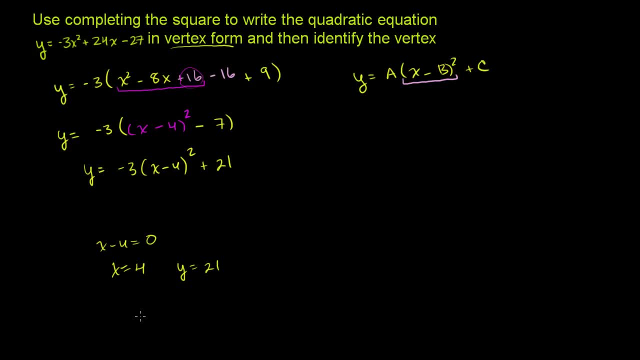 then y is equal to 21.. So the vertex of this parabola- I'll just do a quick graph right here- The vertex of this parabola occurs at the point 4, 21.. So I'll draw it like this: 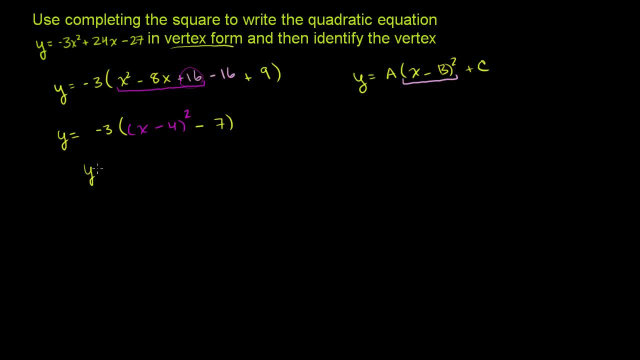 distribute the negative 3.. On to both of these terms. So we get: y is equal to negative 3 times x minus 4 squared, and negative 3 times negative. 7 is positive 21. So we have it in our vertex form. 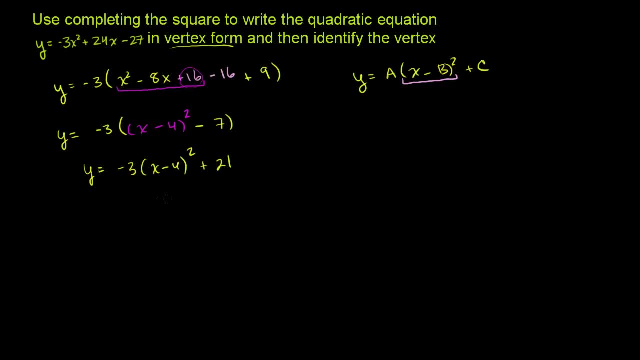 We're done that, And if you want to think about what the vertex is, I told you how to do it. you say: well, what's the x value that makes this equal to 0?? Well, in order for this term to be 0, x minus 4 has to be. 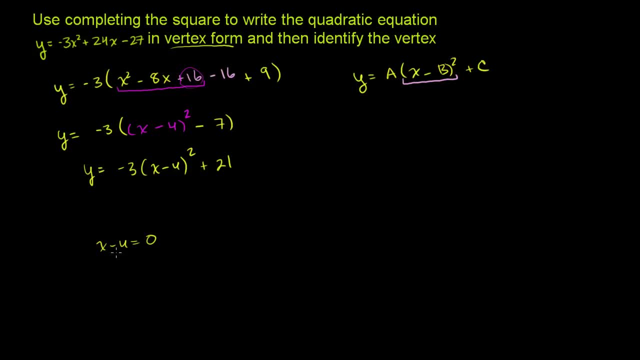 equal to 0. x minus 4 has to be equal to 0, or add 4 to both sides. x has to be equal to 4.. And if x is equal to 4, this is 0, this whole thing becomes 0,. 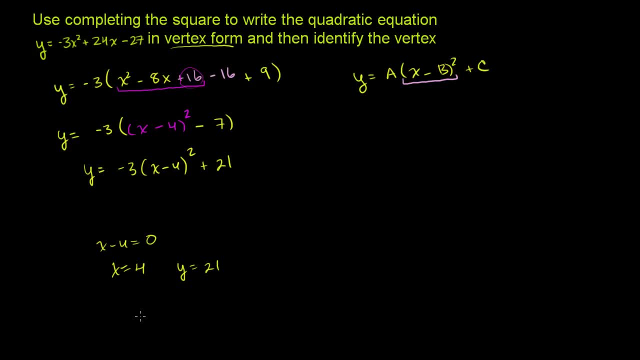 then y is equal to 21.. So the vertex of this parabola- I'll just do a quick graph right here- The vertex of this parabola occurs at the point 4, 21.. So I'll draw it like this: 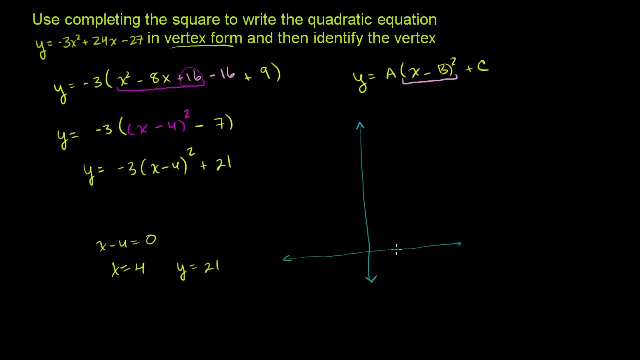 It occurs at the point, If this is the point 4. 4. 4. If this right here is the y-axis, that's the x-axis. So this is the point 4, 21.. Now, that's either going to be the minimum or the maximum. 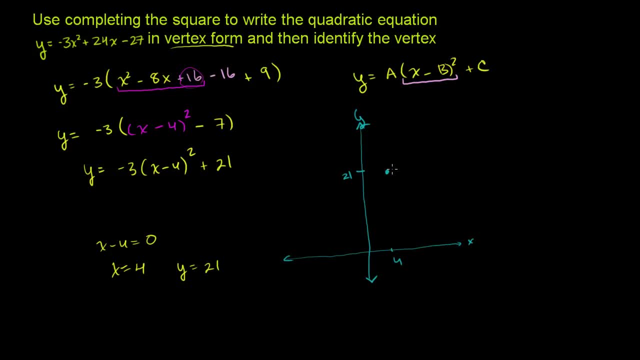 point in our parabola And to think about whether it's the minimum or maximum point, think about what happens. Let's explore this equation a little bit. This thing, this x minus 4 squared, is always greater than or equal to 0.. 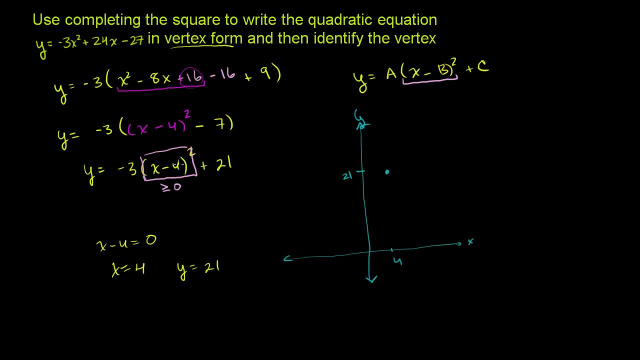 At worst it could be 0.. But you're taking A square, so it's going to be a non-negative number. When you take a non-negative number and then you multiply it by negative 3, that guarantees that this whole thing is going to be less than or equal to 0.. 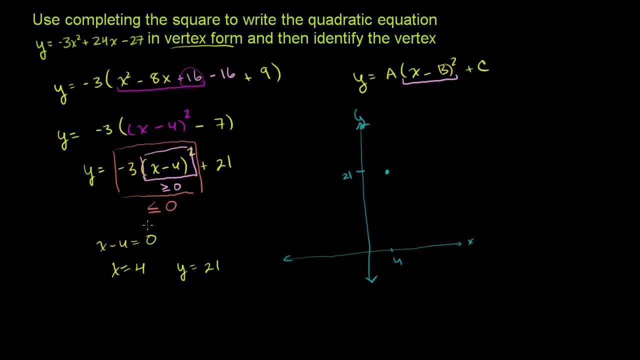 That whole thing is less than or equal to 0.. So the best, the highest value that this function can attain is when this expression right here is equal to 0. And this expression is equal to 0 when x is equal to 4 and y. 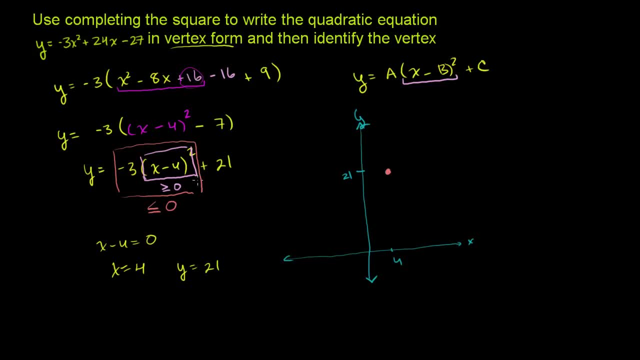 is 21.. So this is the highest value that the function can attain. It can only go down from there, Because if you shift the x around 4, then this expression right here will become non-zero. When you square it it'll become positive. 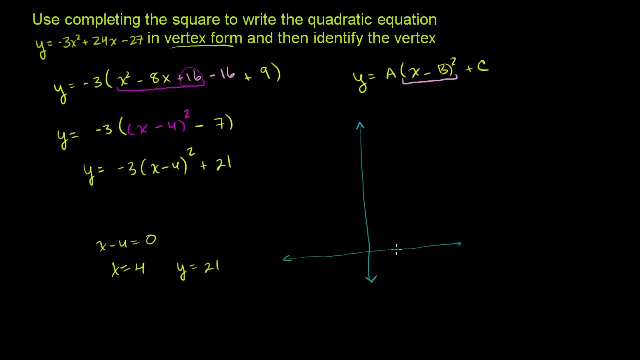 It occurs at the point, If this is the point 4. 4. 4. If this right here is the y-axis, that's the x-axis. So this is the point 4, 21.. Now, that's either going to be the minimum or the maximum. 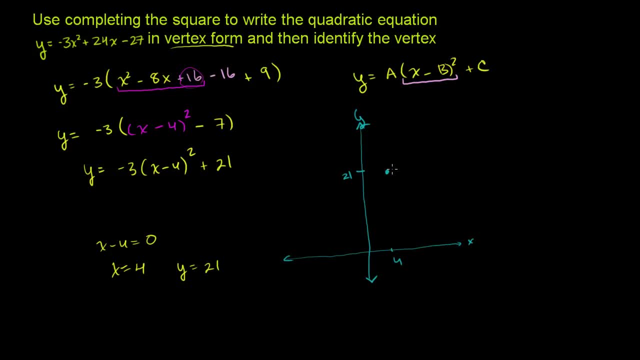 point in our parabola And to think about whether it's the minimum or maximum point, think about what happens. Let's explore this equation a little bit. This thing, this x minus 4 squared, is always greater than or equal to 0.. 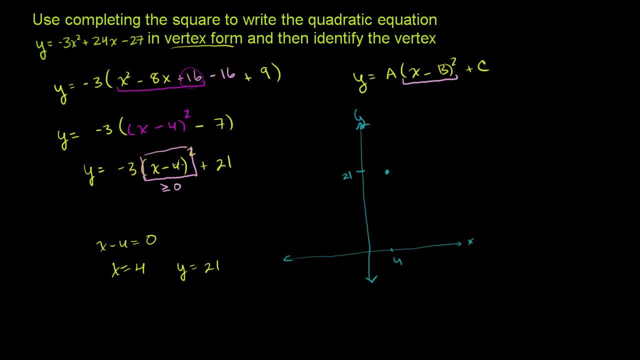 At worst it could be 0.. But you're taking it, You're taking a square, So it's going to be a non-negative number. When you take a non-negative number and then you multiply it by negative 3, that guarantees that this whole. 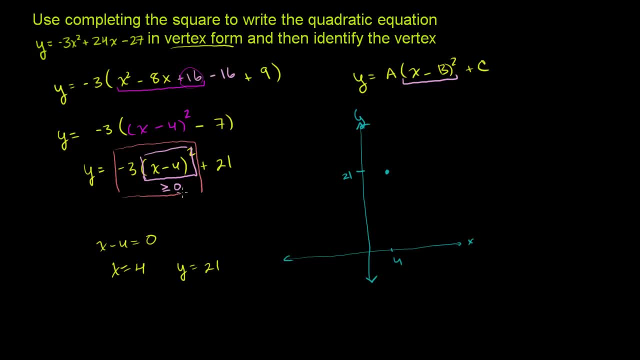 thing is going to be less than or equal to 0. That whole thing is less than or equal to 0. So the best, the highest value that this function can attain is when this expression right here is equal to 0. And this expression is equal to 0 when x is equal to 4 and y. 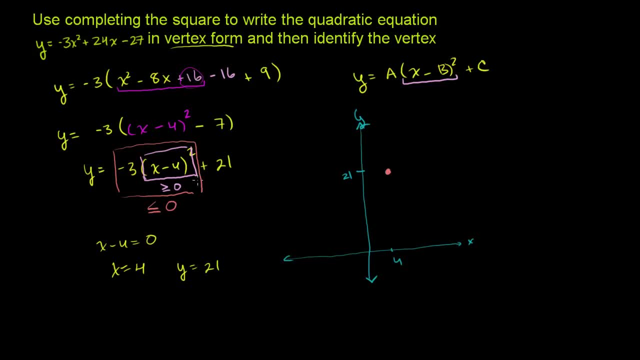 is 21.. So this is the highest value that the function can attain. It can only go down from there, Because if you shift the x around 4, then this expression right here will become non-zero. When you square it it'll become positive. 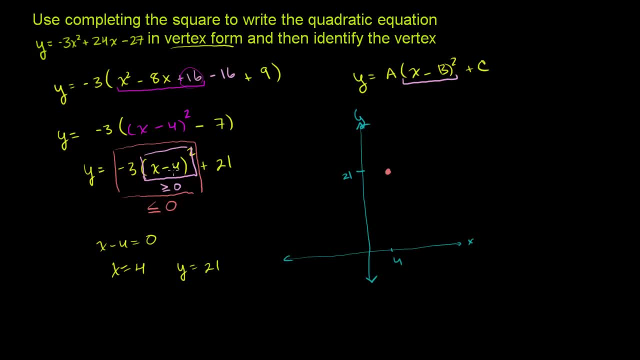 When you multiply it by negative 3, it'll become negative. So you're going to take a negative number plus 21.. It'll be less than 21.. So your parabola is going to look like this. Your parabola is going to look like that. 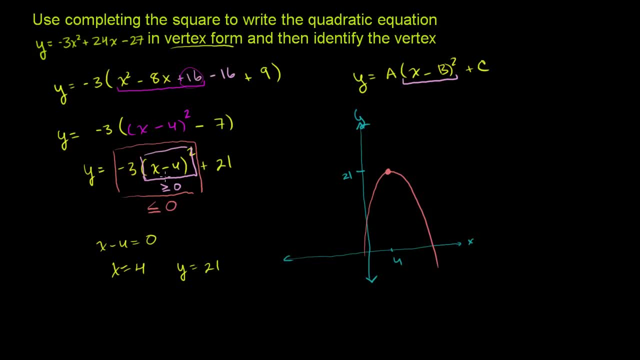 And that's why vertex form is useful. You break it up into the point. the part of the equation that changes in value Say: well, when is its maximum value attained? That's the vertex. That happens when x is equal to 4, and you know its y value. 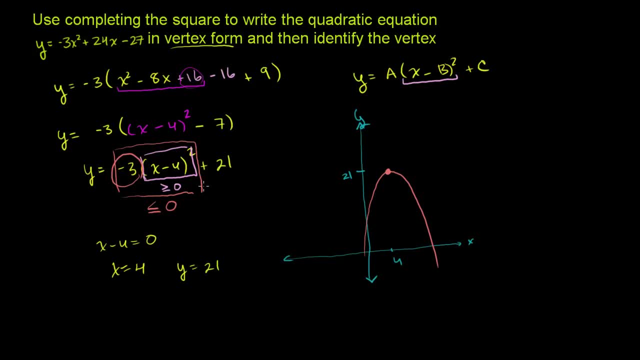 And because you have a negative coefficient out here, that's a negative 3, you know that it's going to be a downward opening graph. If that was a positive 3, then this thing would be at minimum 0, and it would be an upward opening graph.